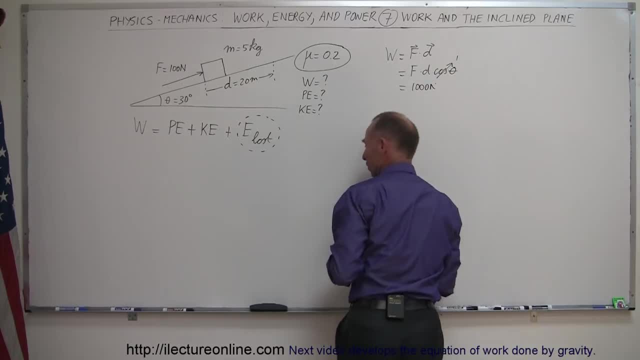 And so we have a thousand newtons, Not a thousand. I think I have only a hundred newtons. A thousand newtons would be a little too much. One hundred newtons of force, One hundred newtons of force, multiplied times 20 meters, which means it's 2,000 newton meters, or 2,000 joules of work done. 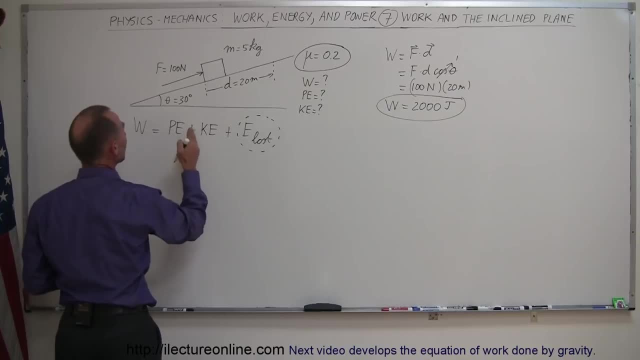 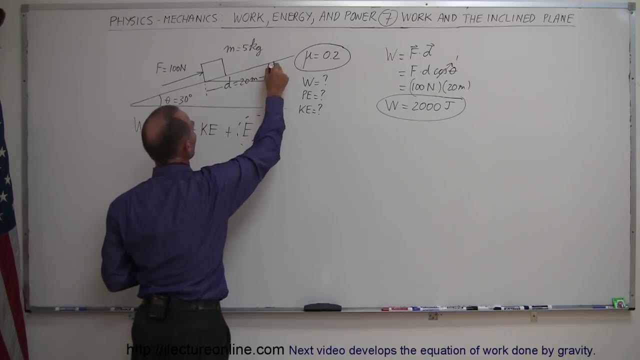 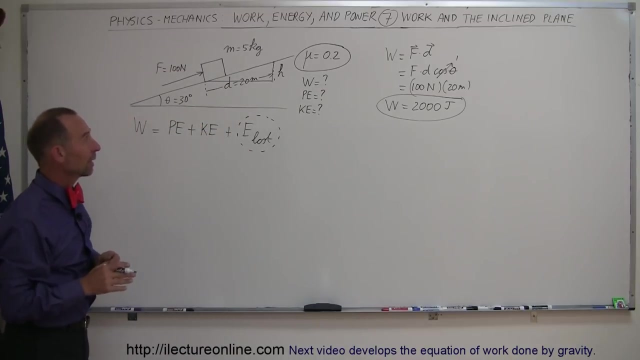 And that work will then be subdivided into potential energy, kinetic energy and energy lost. Now, if we draw a little triangle here, we can then see that this is the height gained by the object by moving it 20 meters along the incline. And let's find out what that height is equal to. 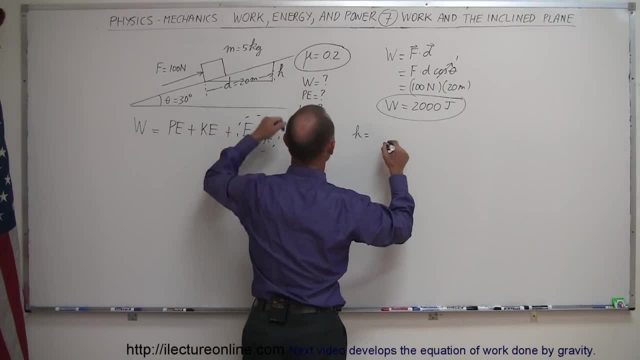 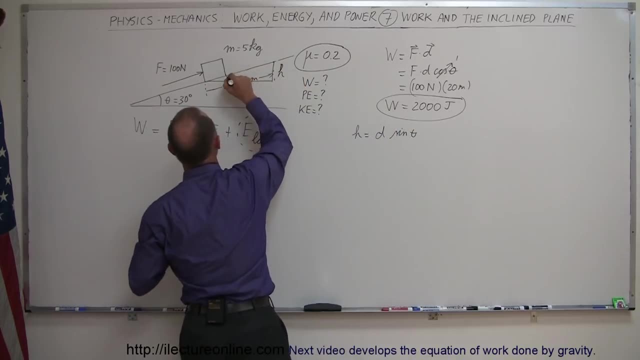 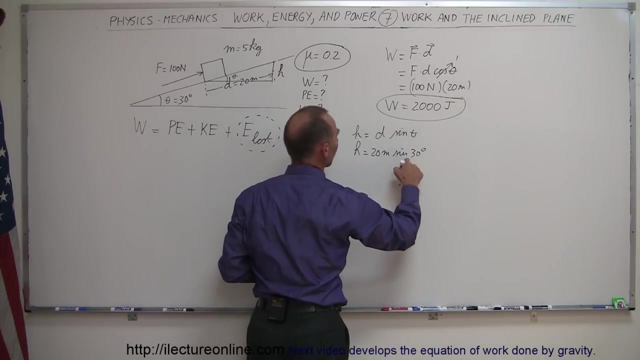 We can say that the opposite side, h, is equal to the hypotenuse d times the sine of the angle theta, Because h is opposite to the angle theta right here. And so we can say that h is equal to 20 meters times the sine of 30 degrees, which is one half. 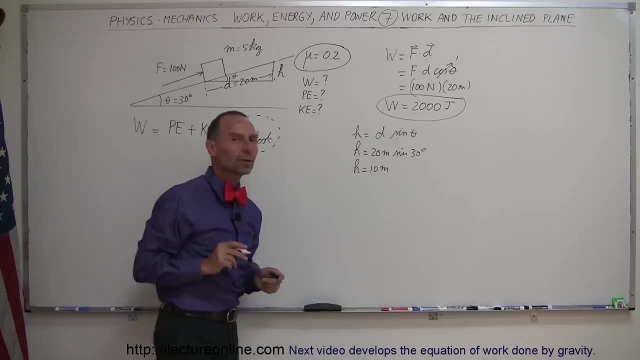 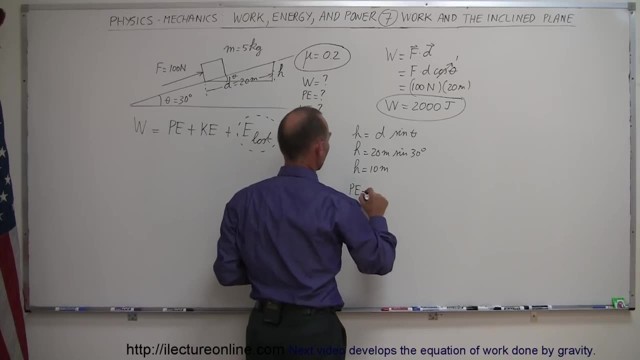 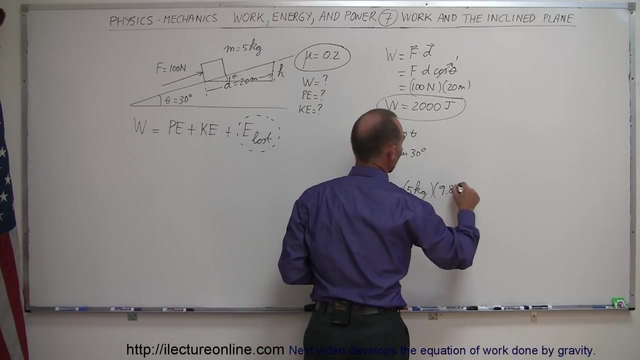 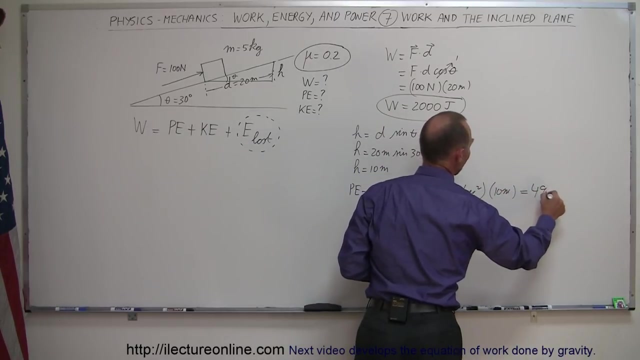 So, therefore, height is equal to 10 meters. Now that we know the height, we can figure out the potential energy gained by this object. This object will gain potential energy equal to mg, Which is 5 kilograms times 9.8 meters per second, squared times the height of 10 meters, which is a total of 490 joules. 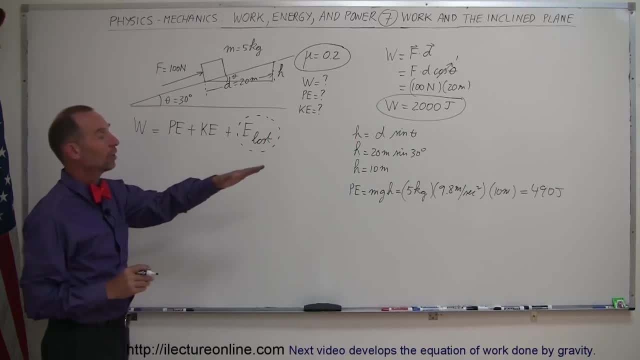 So out of the 2,000 joules of work done on the object, 490 of it is utilized to give it the additional potential energy by gaining a height of 10 meters. Now how much energy is lost due to overcoming the friction? So in order to figure that out, we need to find out what the friction force is. 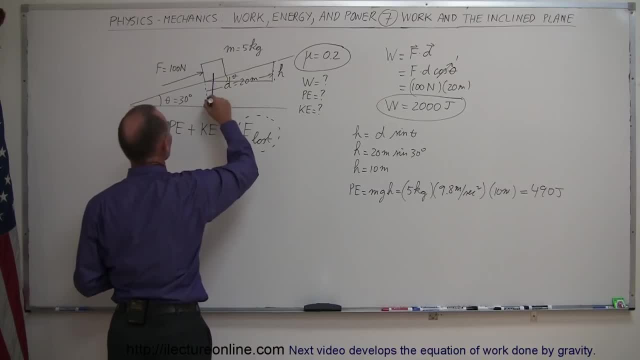 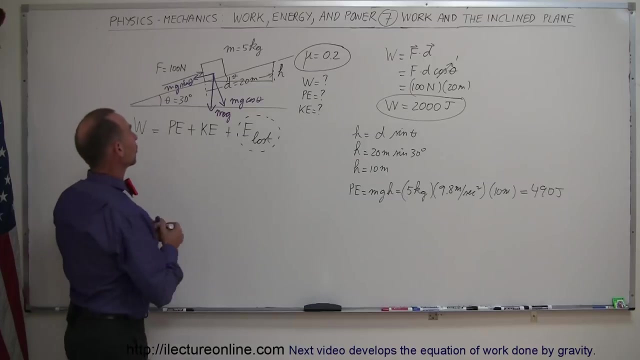 So we can see here that this is the weight of the object, mg, And this, of course, would be the perpendicular component, mg cosine theta. This is the adjacent component, mg sine theta. Now we have the normal force pushing back right here, And the magnitude of the normal force is equal to mg cosine theta. 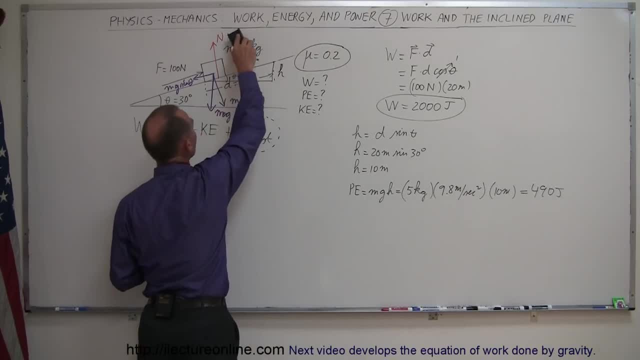 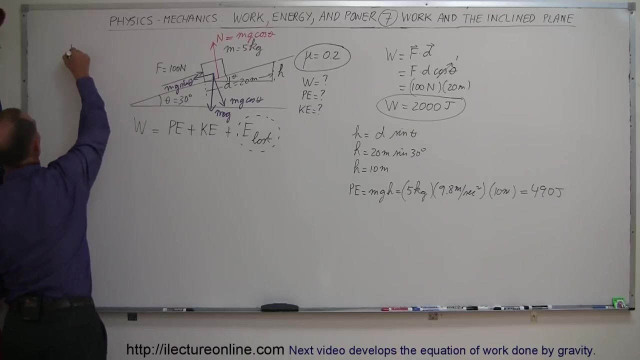 So that's equal to- I forgot my little equal sign. So this is equal to mg cosine theta. And then the friction force, of course, is equal to the normal force times mu. So let's go over here. So the force friction, which by definition is the normal force times mu. 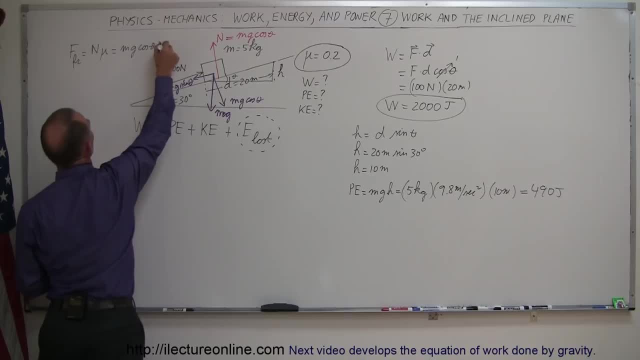 Which would be equal to mg cosine theta times mu. Let's figure out what that is equal to. Alright, so in this case that would be the mass of 5 kilograms G of 9.8 meters per second squared Cosine of theta would be cosine of 30 degrees. 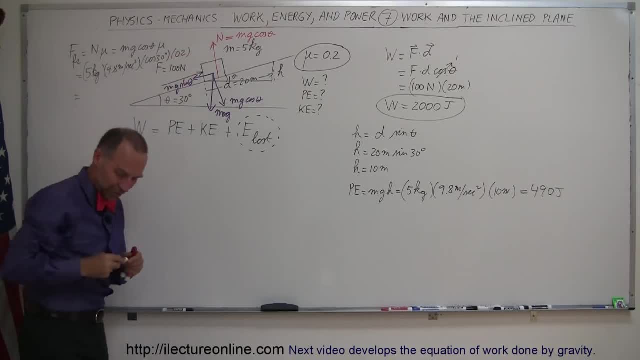 And the mu of 0.2.. So let's find out what the strength of that friction force is. So we have, 5 times 9.8. Times, the cosine of 30. Times 0.2. So we have a force of 8.5 newtons. 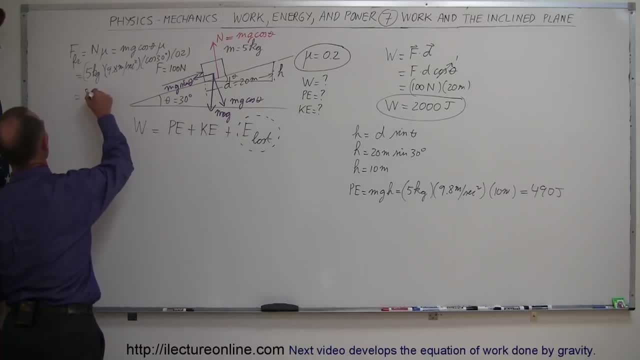 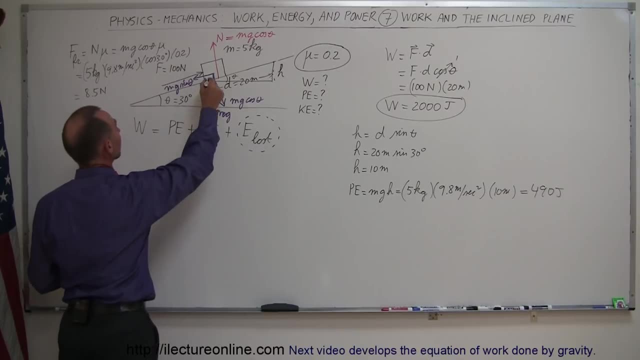 That's close enough. Alright, so we have a force of 8.5 newtons. Now notice the friction force is going to be pointing in this direction. So let me note that. So here we have force friction and it's in a negative direction. 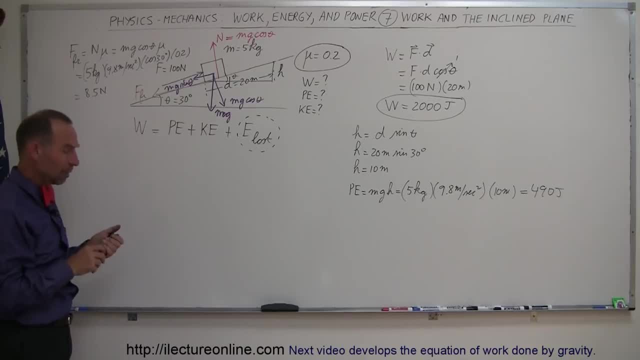 Now, if we're going to calculate the work done by overcoming the friction, We can say that, of course, work because of friction Is equal to The force of friction. times the displacement And notice. these are vector quantities, But in this case the friction force is pointing in this direction. 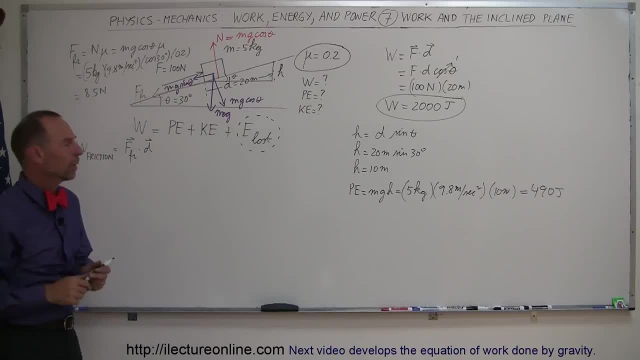 And the displacement is in that direction. That's 180 degrees apart, Which means that this is equal to the magnitude of the friction force Times, the magnitude of the displacement Times, the cosine of 180 degrees, Which, of course, is a negative 1.. 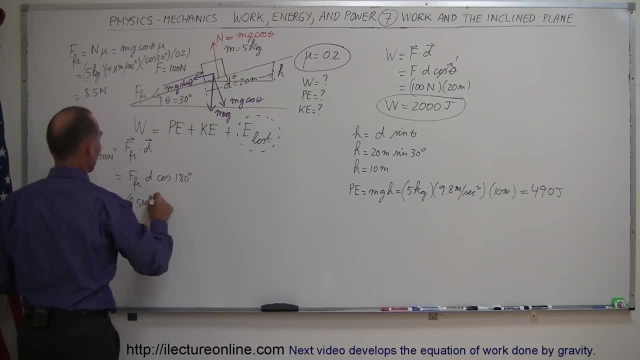 So this is equal to 8.5 newtons Times a distance of 20 meters, Times the negative 1.. So this is equal to 170 newtons, of course, And negative 170 newtons, Which is the work done by the friction. 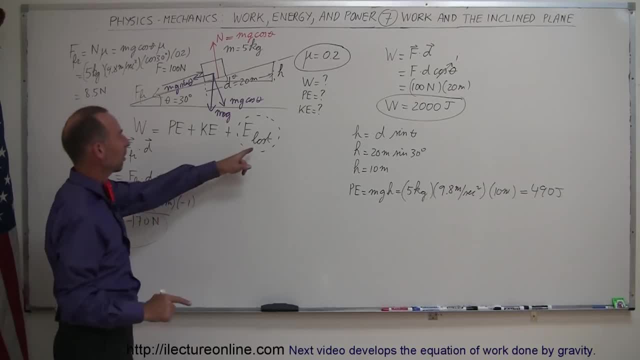 This is the energy loss part that we're talking about here, So not all of the work was put into potential kinetic energy. Some of it- 170 newtons of- Oh, not newtons Newtons- is force. I need joules- 170 joules of it was lost- to overcome friction. 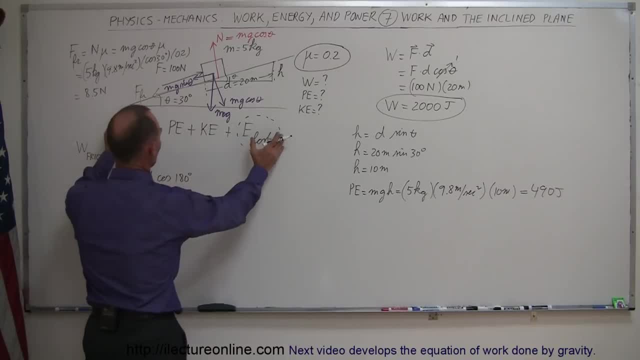 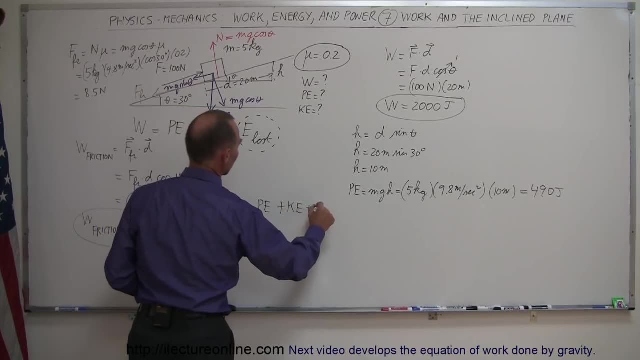 And so That means that When we take this equation right here, We have the work done, Which is equal to the potential energy Plus the kinetic energy Plus the energy lost, And so the work done right here, Which is 2000 joules, 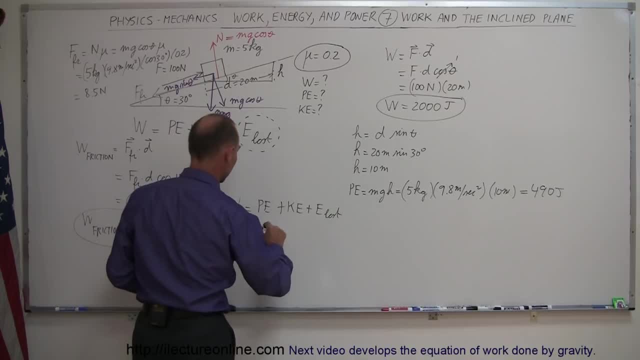 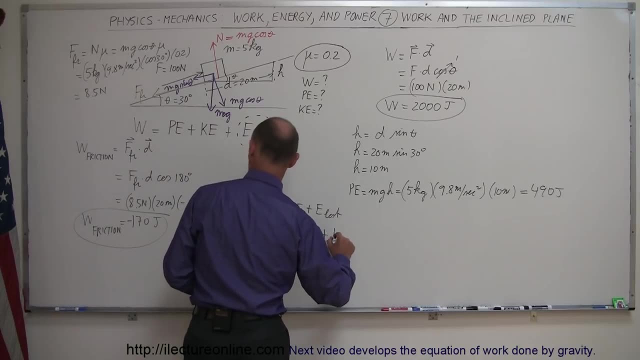 Is equal to the potential energy, Which we calculated to be 490 joules, Plus the kinetic energy, Which we haven't calculated yet, Plus the energy lost of 170 joules. And I say, well, Don't you have a minus here? 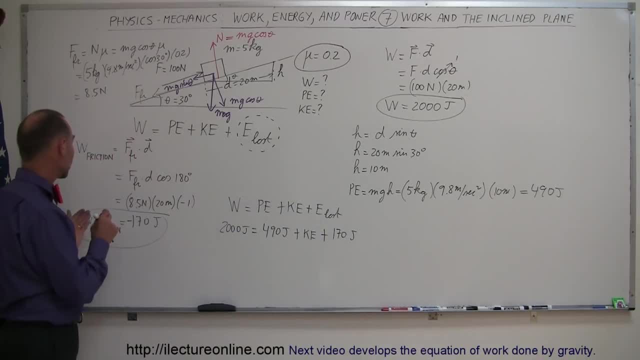 Why do you make that a plus? Well, the minus simply means That's the work done by the friction, Which needs to be subtracted from the work done on the system To balance out the equation. So therefore we have to add it. 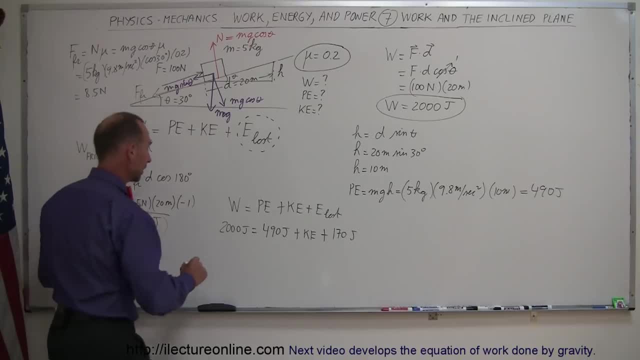 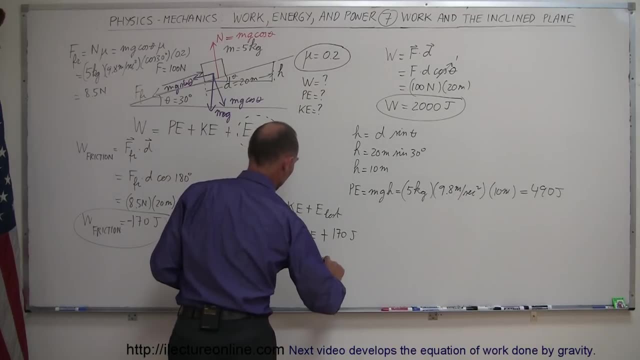 To the right side of the equation. That means I can now calculate my kinetic energy. So my kinetic energy Is equal to the 2000 joules Minus the 490 joules, Minus 170 joules, So that 590.. 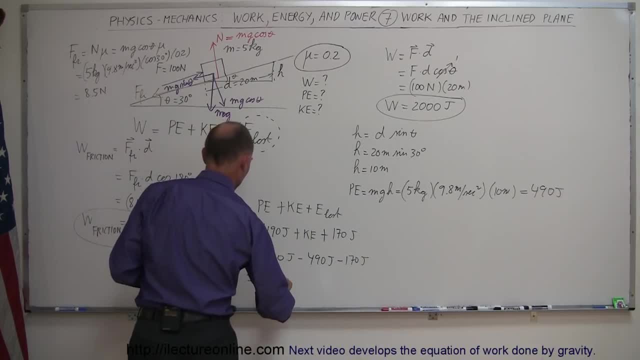 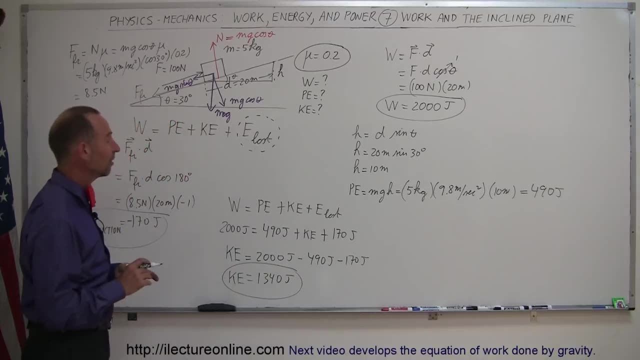 That's 660.. That means 1340 joules of kinetic energy Will be given to the system. Now, At this point, Let's say I want to know What my final velocity is of the object When it reaches a distance of 20 meters. 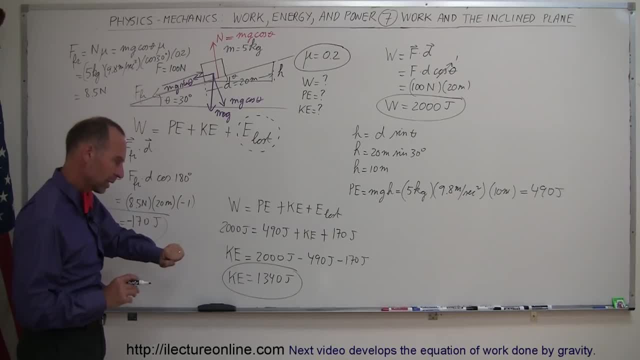 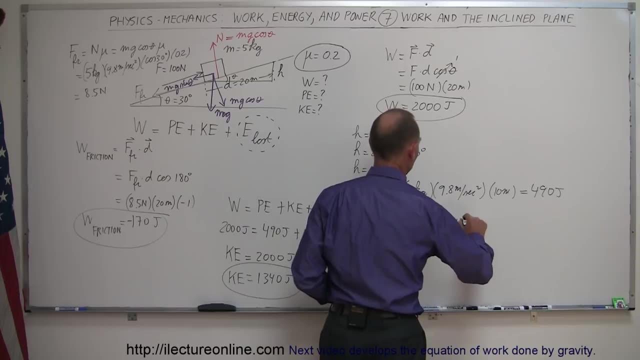 Since I now know my kinetic energy And this quick calculation- I think I did that correctly- I can say kinetic energy Is equal to 1 half mv squared. So multiplying both sides by 2. And divide both sides by m, I get v squared. 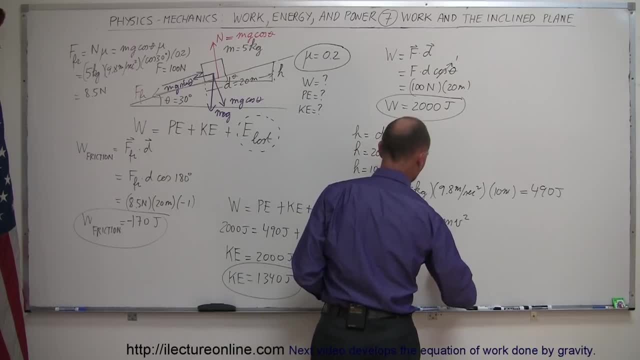 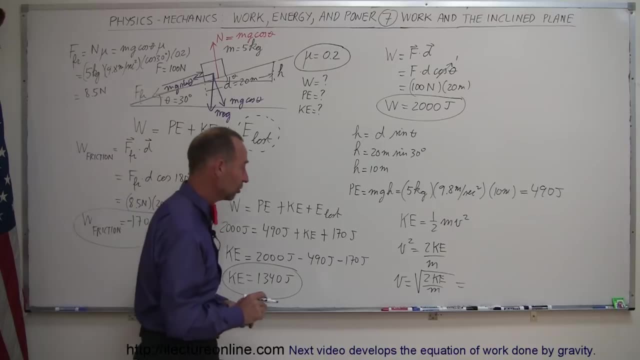 Is equal to 2 times the kinetic energy Divided by the mass, Which means The velocity is equal to the square root of that, Which means If I now plug in The kinetic energy and the mass Into that equation, 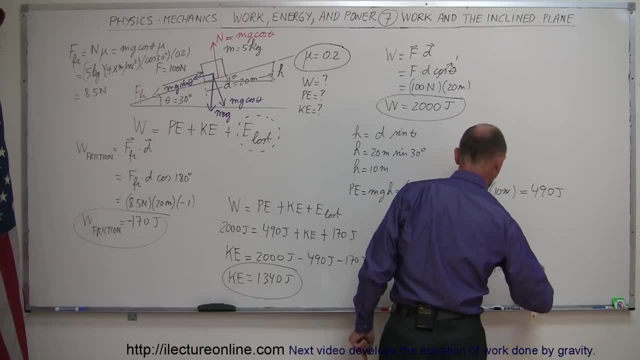 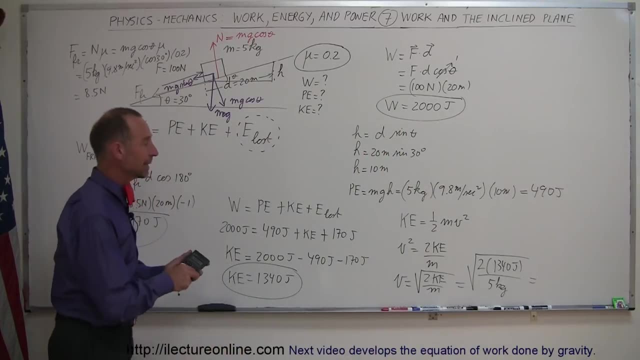 2 times 1340 joules Divided by the mass of 5 kilograms. Take the square root, I now have the velocity Of that block At the end of that 20 meter journey, So 1340.. Times 2.. 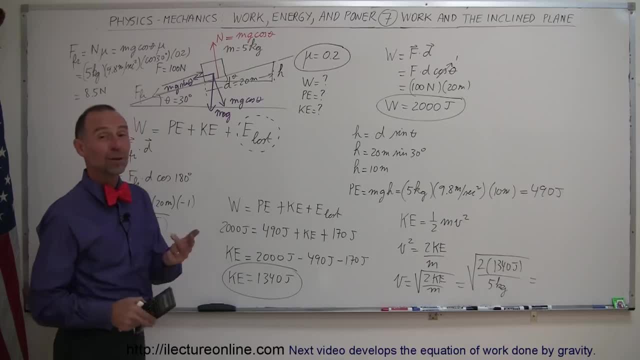 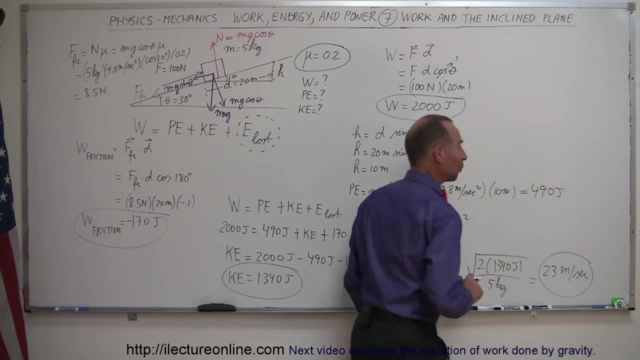 Divided by 5. And then taking the square root of that And would be 23.15.. Just call it A velocity Of 23.. Meters Per second And there is a really nice example Of how.